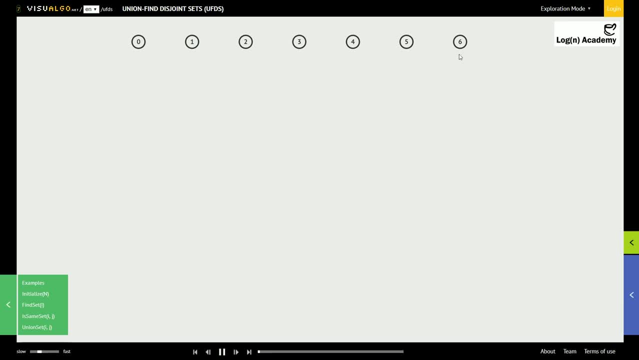 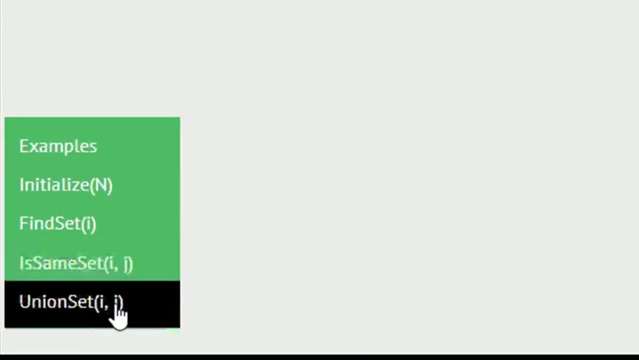 So, as you can see, here I have zero to six elements, So these are sets, and these sets containing only one element, right? So now let's do the, let's perform the union operation. So here I have two values, i and j, So I can here give the number, that which set I want to join. 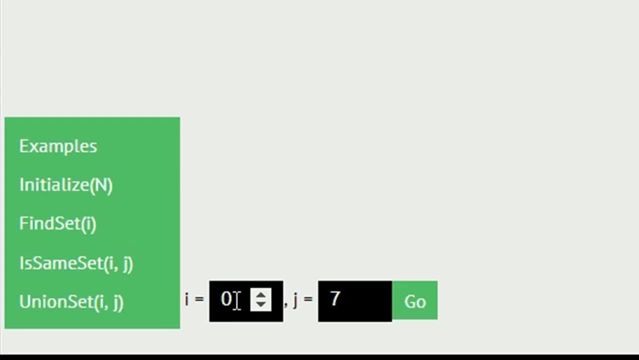 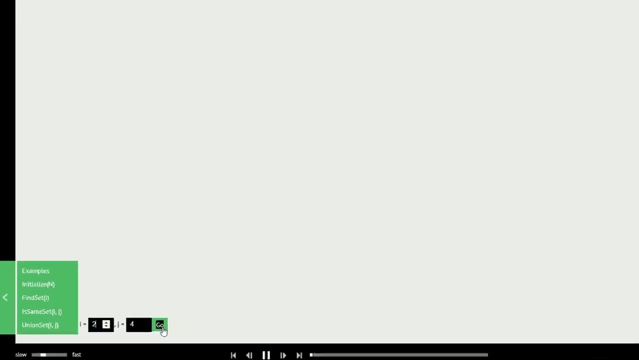 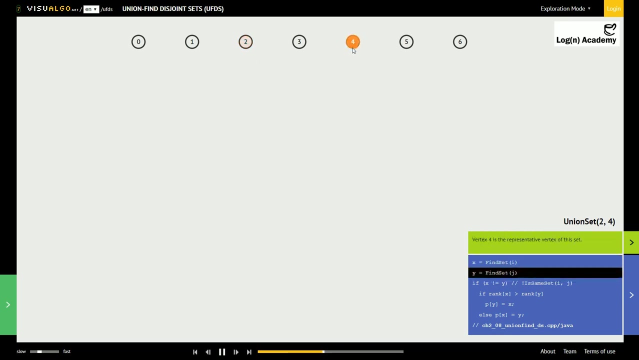 Which two disjoint set. I want to union. So let's say: first I will say two and two, and let's say four, I want to union two and four. So as you can see here, two, it has found two and it has found four, and then it will join them. 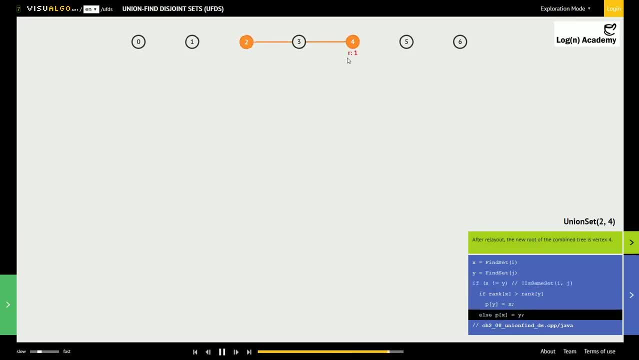 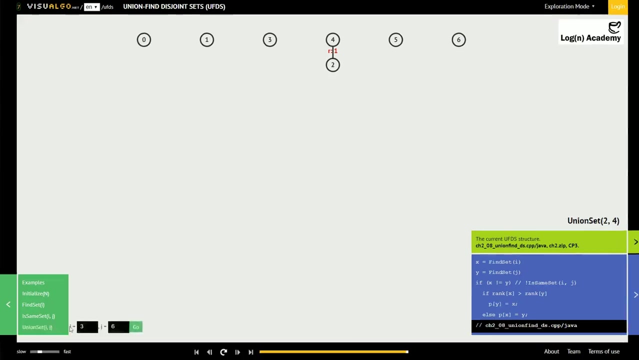 So this is the final result. So here, on the right hand side, this is the algorithm, which is which is working, and it's showing the movement of the, of the lines, the execution of the line. So now let's union. now let's union three and five. 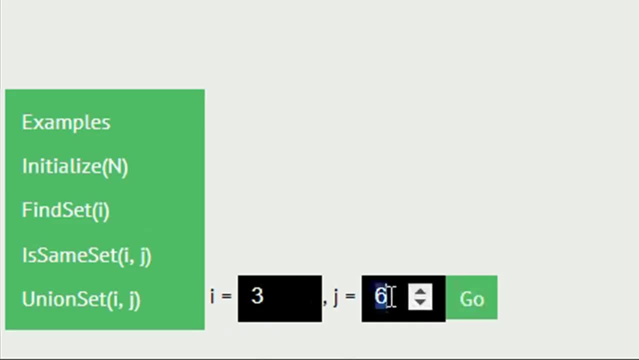 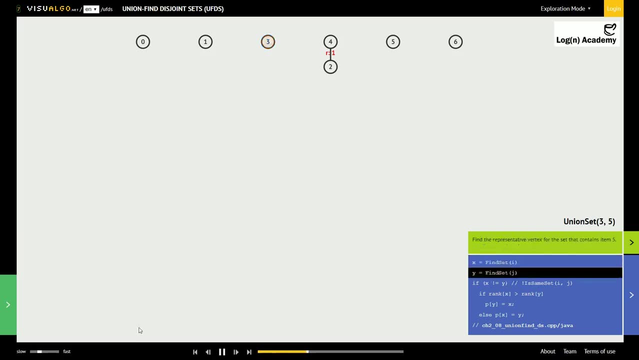 Okay, let's union three and five. So I have three here I will say five, And now it's going to group three and five. So it has found both elements. Now it's a union and here in this, in the first set, four is the representative, or you can see, the four is the root node, and same on the second set. 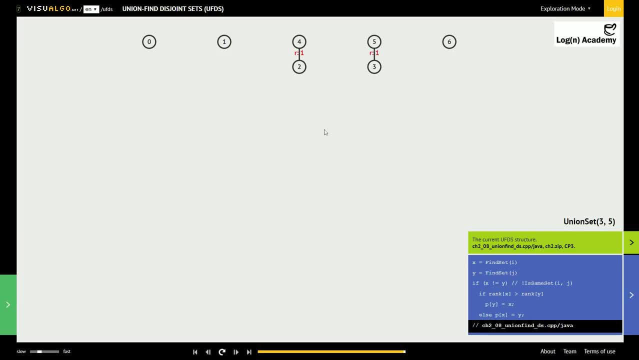 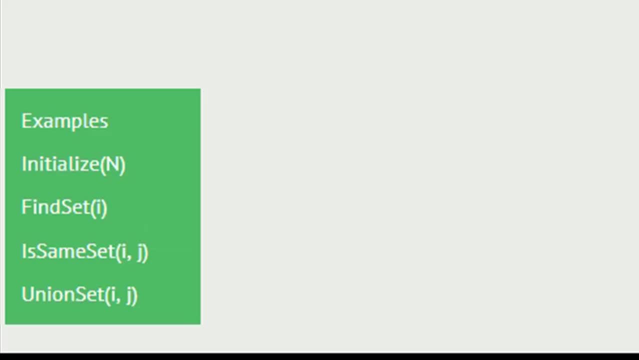 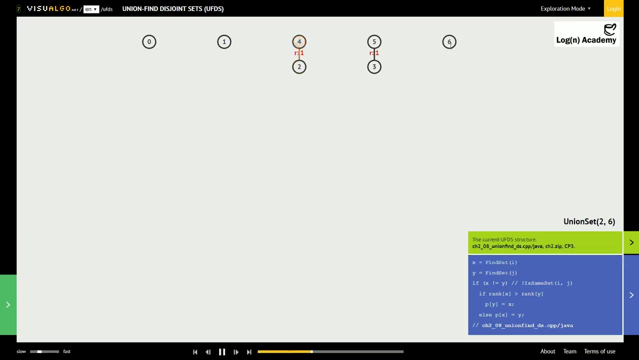 We have five as a representative of this whole set. Okay, now let's union. Let's union two and six. Okay, we have two here and we have six here. Now let's union two and six. So two: two's root node is four and six, six is is the individual node. 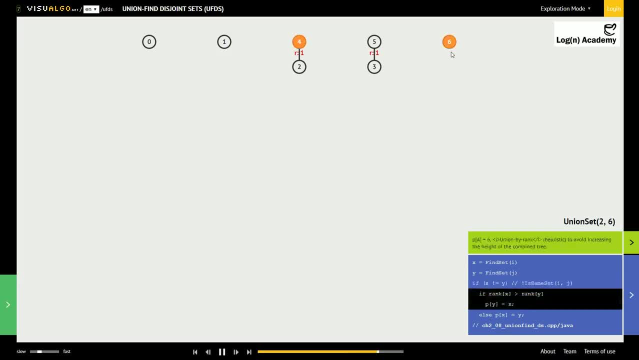 It's the it is itself is a root node. So it will combine these two, four and six, Right? Okay, Now Let's combine One zero and one. Let's do zero and one, Zero and one. So here we have zero, and then we have one. 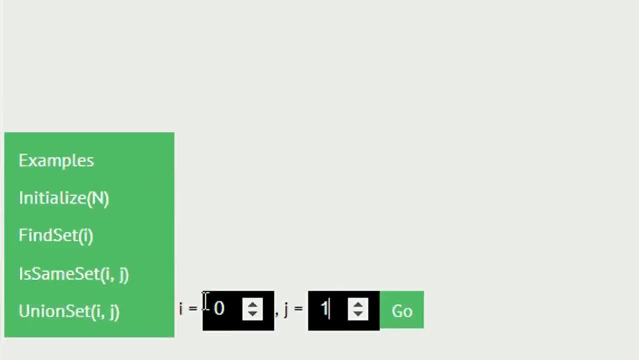 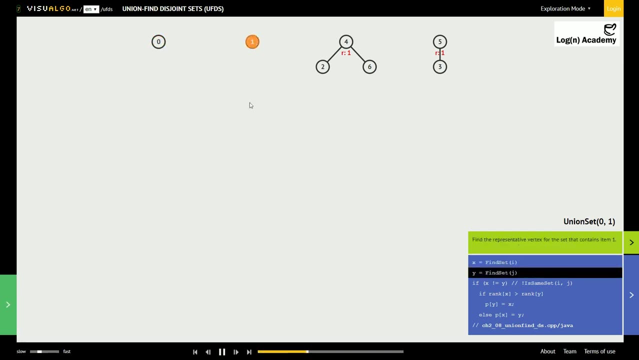 And then it will unite these two. So let's do zero and one, Let's do zero and one. So here we have zero And then we have one, And then it will unite these two And it will make, I guess, one will be the root node. 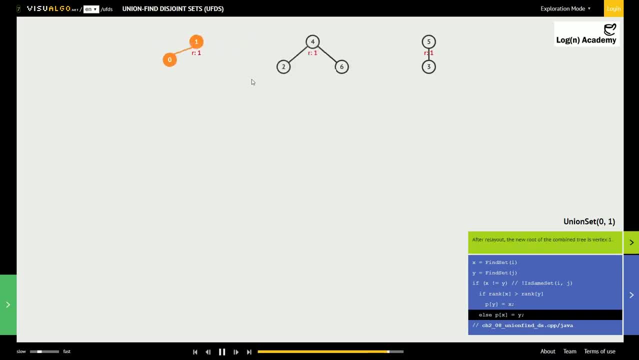 And then it will make, I guess, one will be the root node. Yeah, It is making the greater values as the root node. Yeah, It is making the greater values as the root node. Yeah, It is making the greater values as the root node. 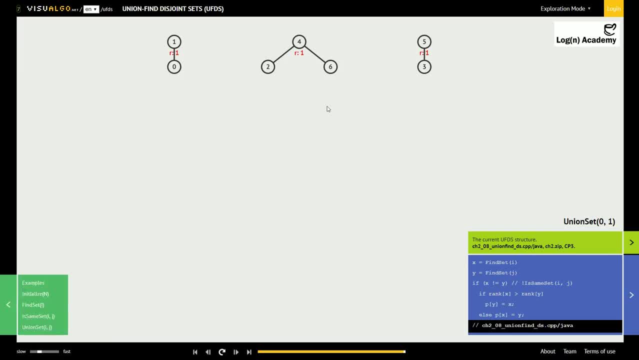 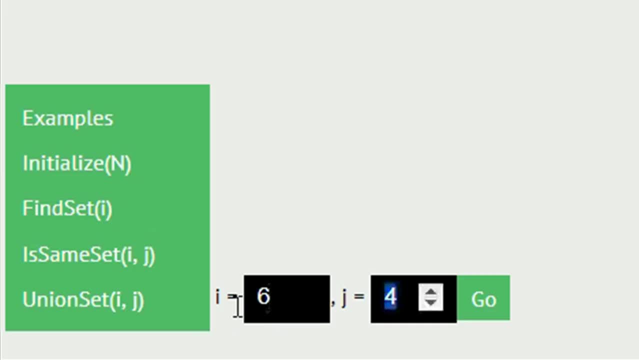 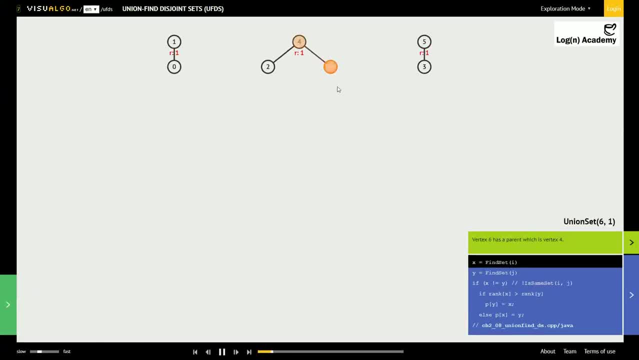 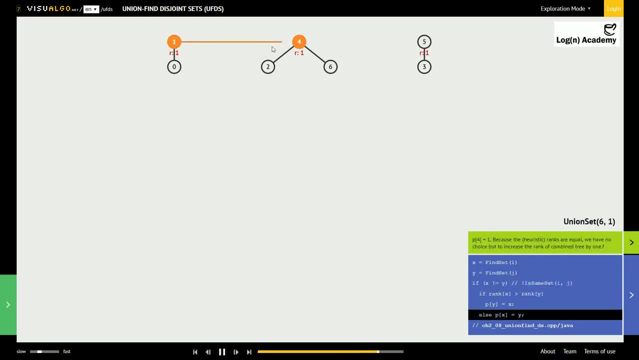 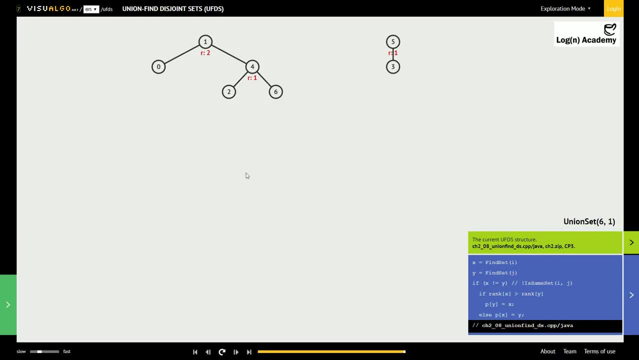 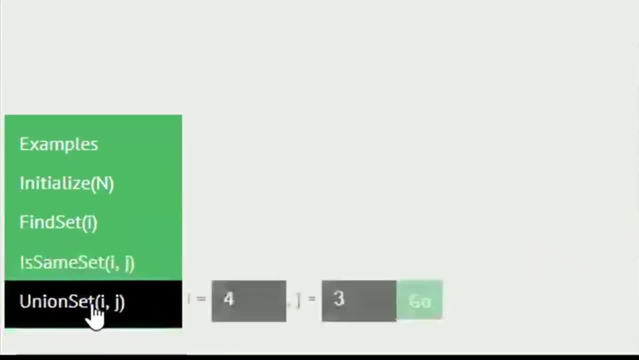 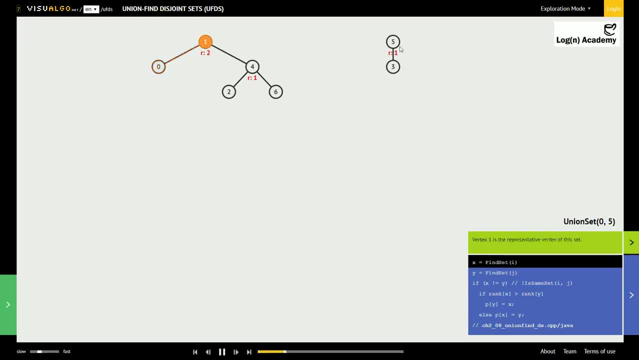 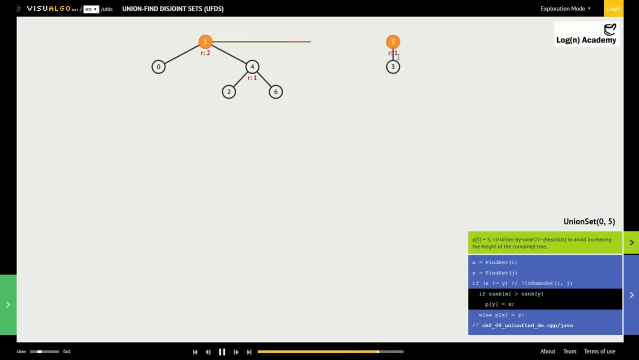 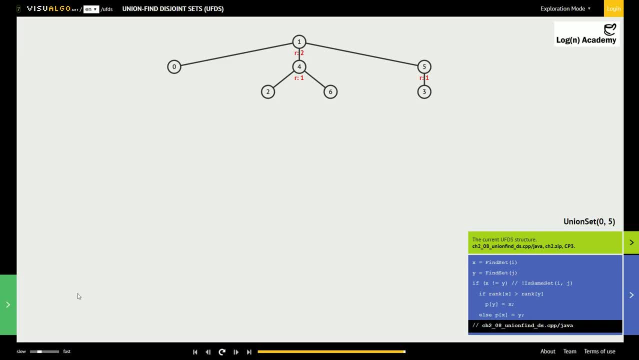 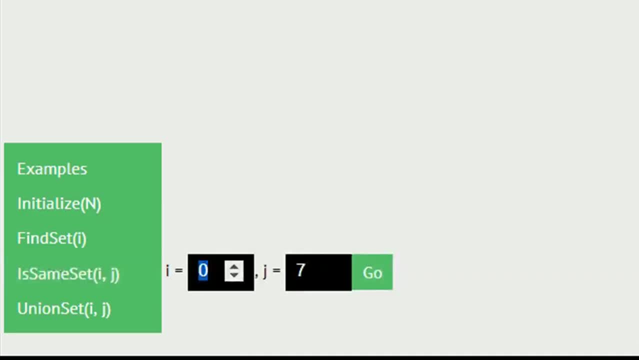 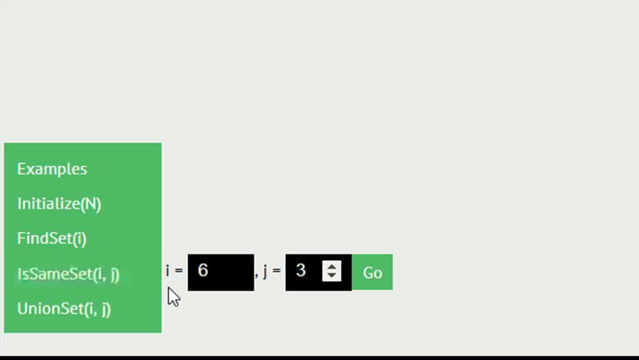 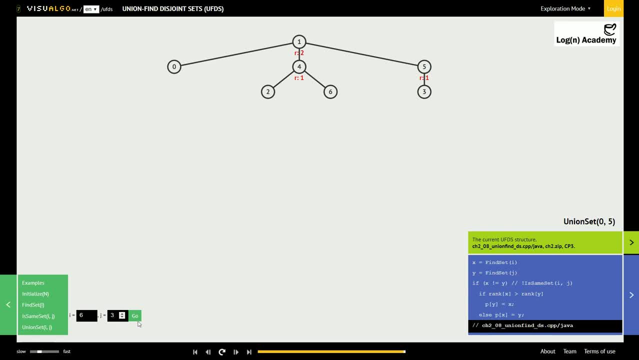 So now it will make connection one and four rotation right. we headed it six, six root is four and the four root is one, and now you see it has compressed the path. and three, threes root is five and five root is one, and now it will apply the compression with three right. so now both. 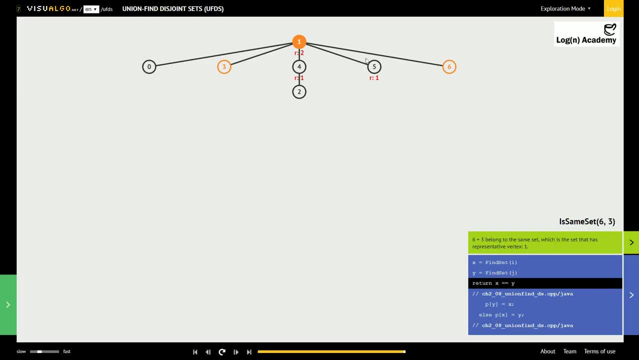 three and six are directly pointing to one. it is applying path compression on find method. right, so here we have used is same set and when it, when using this method, when we call this method, it checks that is there any node which which has which needs to be combined to the root node, which which any node on? 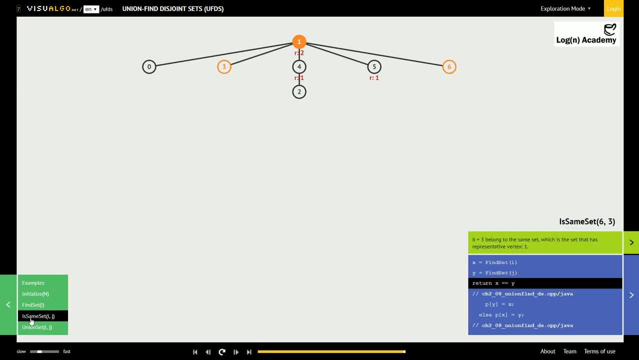 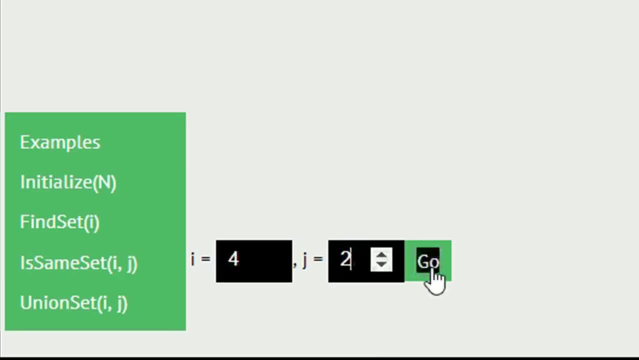 which path compression can be applied so that this method applies the compression on that, on that node again, same way we can do with with four and two, so I can say four and two and it will check that. is there a node between in in this screen which needs to be? 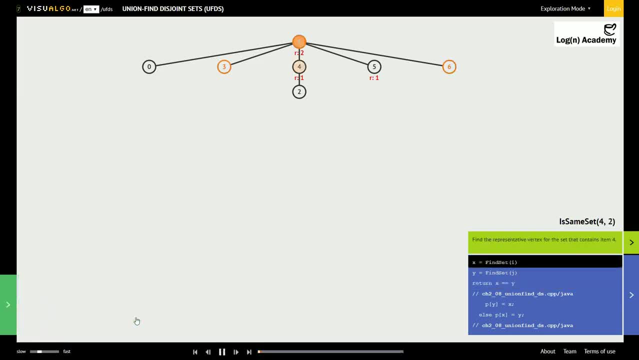 compressed, and it will do the compression for four. root is one, that's fine, and then it will check for two. now the tools: no, root is four, and then it's one. so now this is the candidate for compression, two is the candidate, and as you saw it,